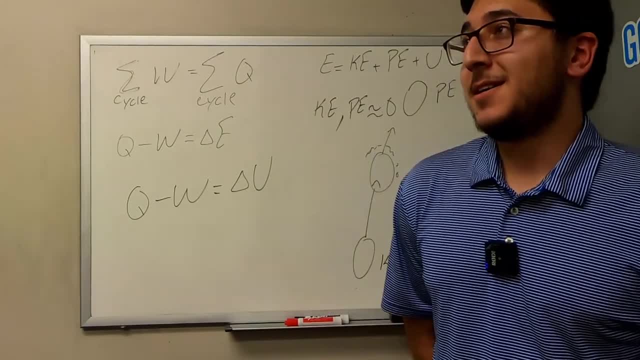 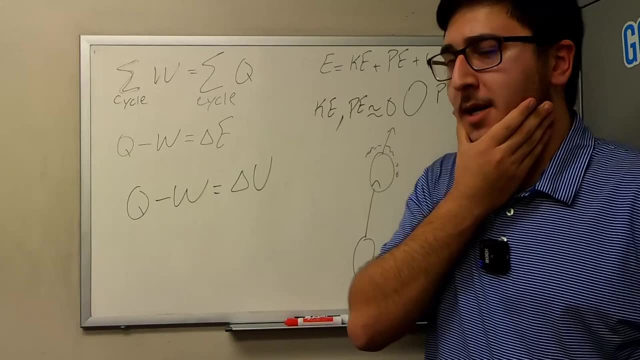 What advice do you have for thermomajors? Okay, an advice would be: is it's a lot of material, Like our first exam is coming up in nine days, Okay, And it's only three chapters. It might not sound like a lot, but three chapters of thermodynamics. 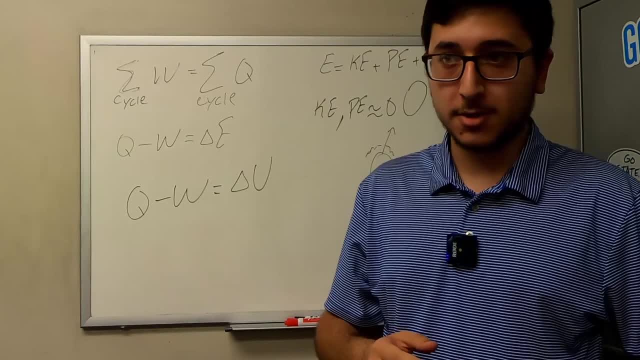 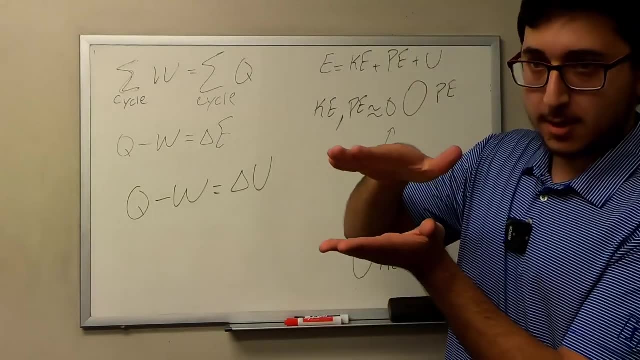 is basically equivalent to seven chapters of a regular calculus book. Wow, Yeah, it's over, like at least I would say, 300 pages, just the three chapters. Yeah, our book is like this thick. Wow, And that's only three chapters covering the introduction to thermodynamics. 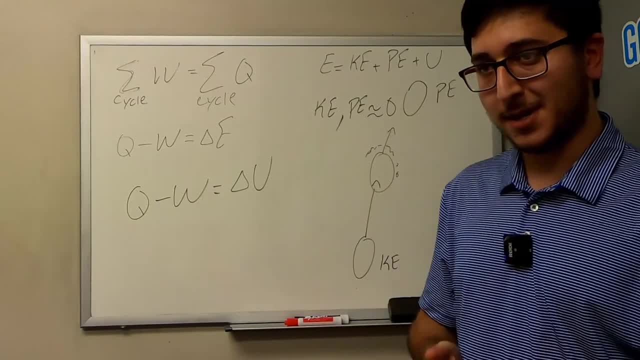 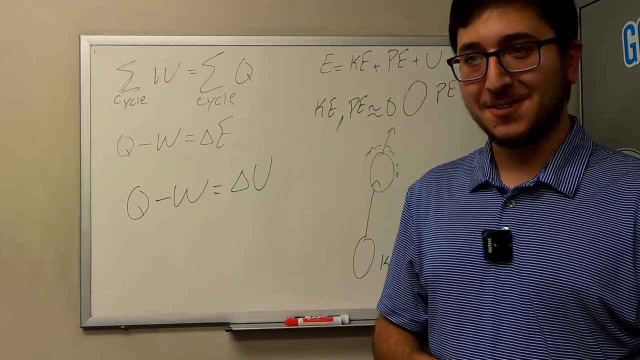 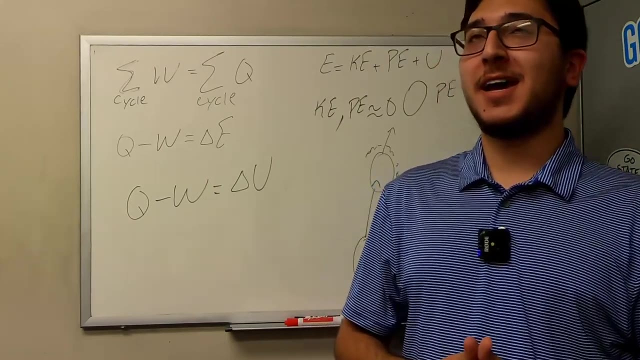 We haven't went to deep stuff like analyzing full engines and systems interacting with the environment. Yeah, so just do your homework and stay on track How many people are in your class. We have a full class- almost 300, 350 students. 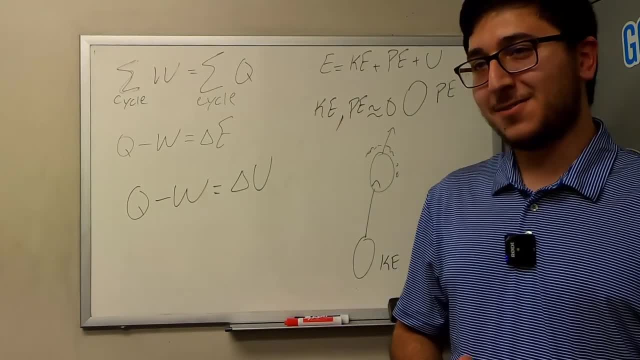 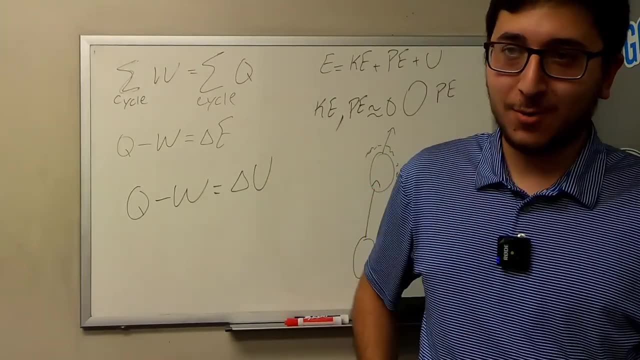 How many are left? We probably lost like 25 students. It's not much. After the exam. are you guys going to go long After the exam? yes, Yeah, I realized that in my previous engineering classes. after exam one we lose like a quarter of the class. 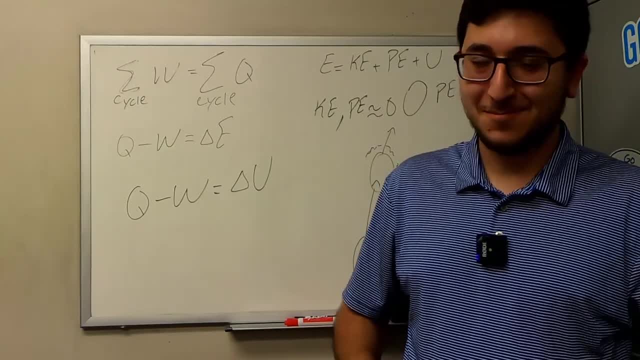 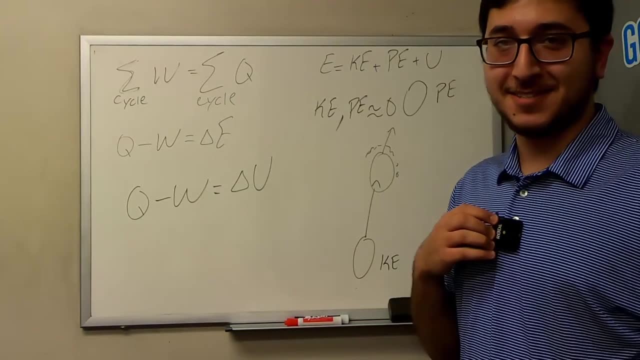 Yeah, Yeah, Cool, Awesome. Well, thank you, You're welcome. Okay, Yeah, what's your major again? Aerospace engineering, Aerospace, Yes Yeah, so still a long way to go. Still computer engineering, Still computer engineering. 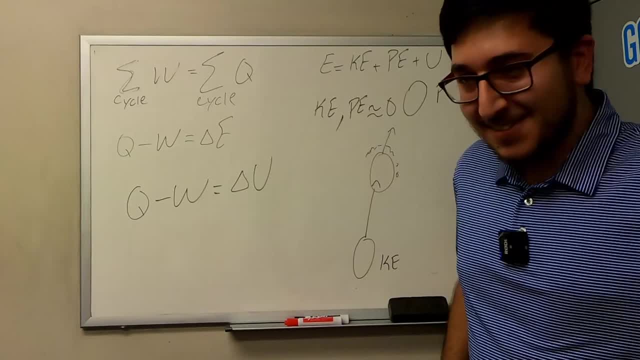 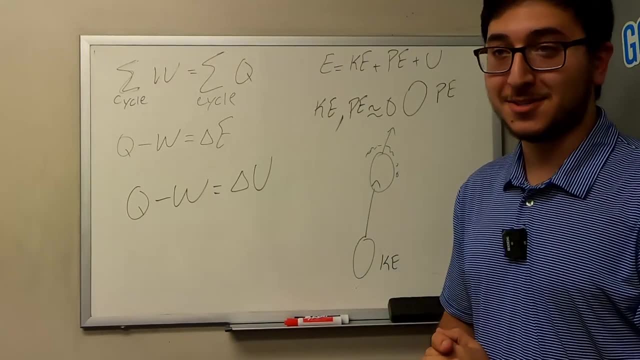 Yeah, I'm full in math. I'm dead. No, it's not that bad. actually, I would say engineering is easier than math and pure physics. You think so? I think so, yeah, Really Yes, I do Why. 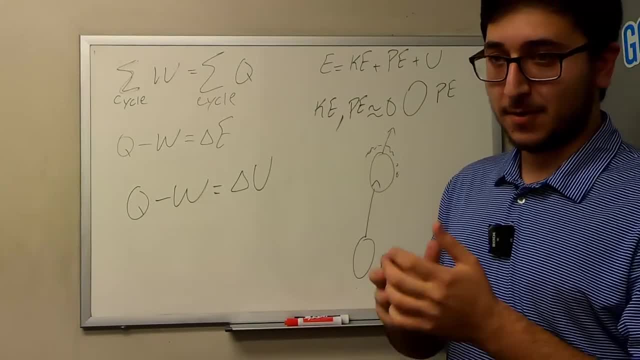 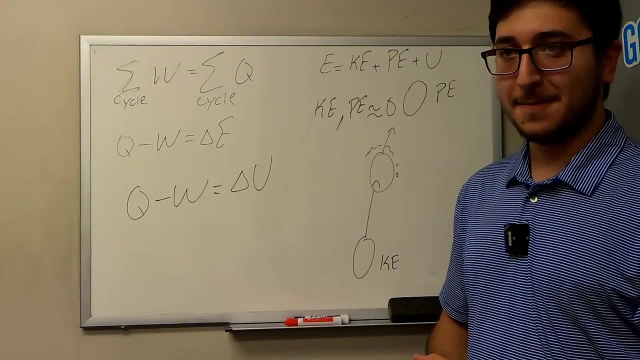 It's not a lot of complex math that we have to do. And the concept? if you actually read the book and understand it, it's easier. But isn't that harder than like just doing an integral? Well, I can do an integral and then understand the concept and derive the integral. 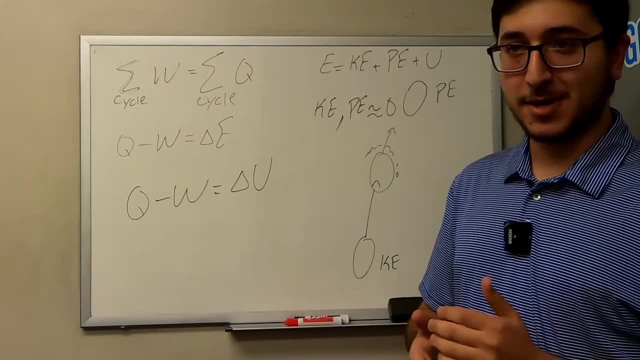 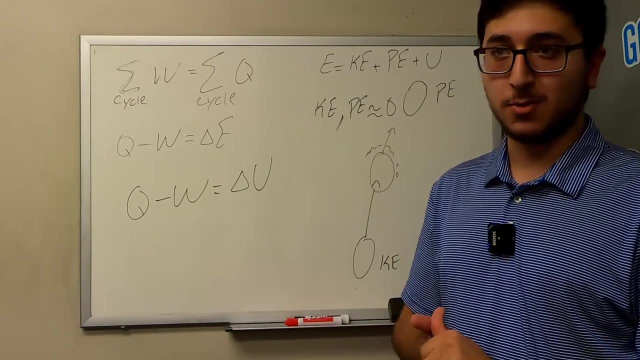 Sure, Yeah, Yeah, Like in dynamics. right now We don't have, we don't actually memorize equations. We derive an equation based on the system that we have and that will be based on a figure or the chart that we get.